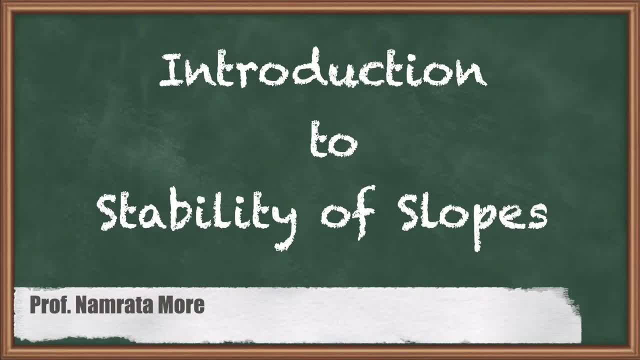 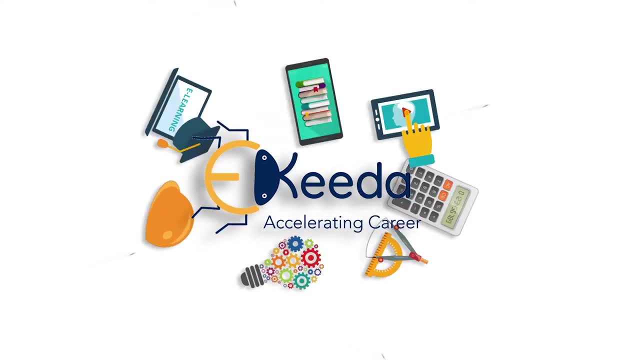 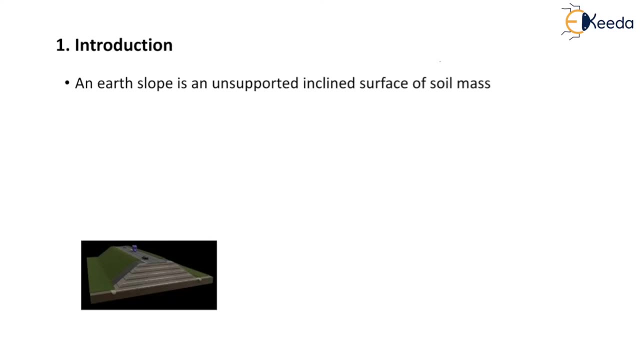 Hello everyone, in this video I am going to introduce you the chapter stability of slope. An earth slope is an unsupported inclined surface of this soil mass. So this is, suppose, elevated ground surface. then on the either side there is inclined surface. This inclined surface of the soil is called as slope. This slope is provided or these earth slopes are. 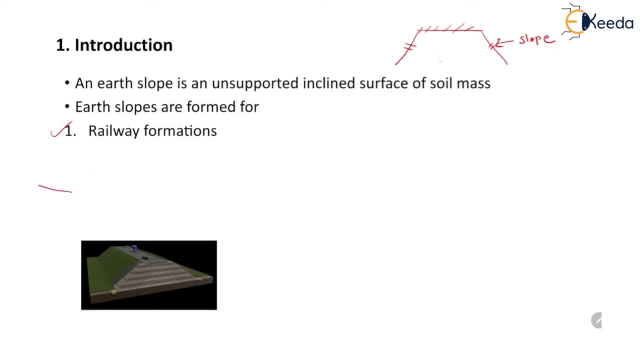 formed for first railway formation. So here in this image we can see that the railway track is at higher elevation than the actual ground surface. So for this railway track, the ground surface is at higher elevation than the actual ground surface. So for this ground surface, the ground surface is at higher elevation than the actual ground surface. 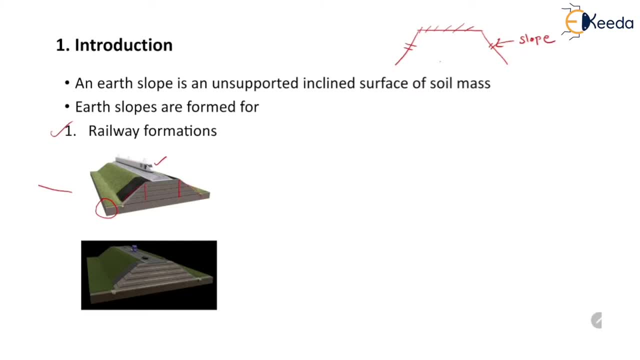 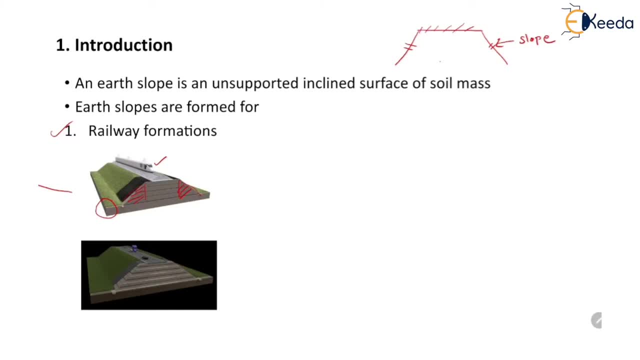 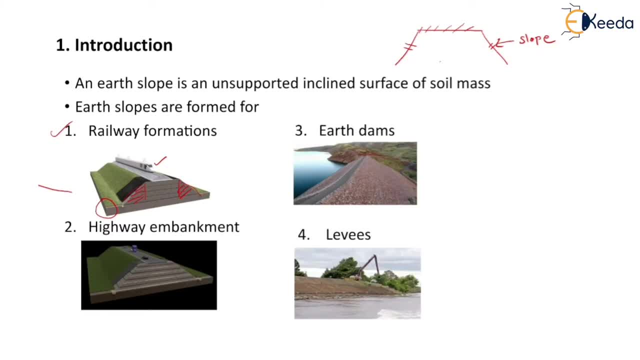 track, the ground surface is at higher elevation than the actual ground surface. So for this railway track, the ground surface is at higher elevation than the actual ground surface. So for this railway track, the ground surface is at higher elevation than the actual ground surface. So for this railway track, the ground surface is at higher elevation than the actual 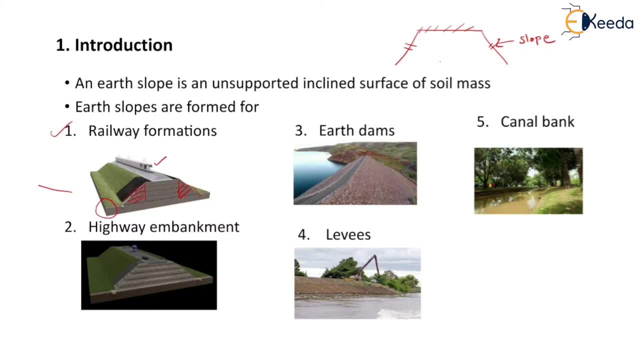 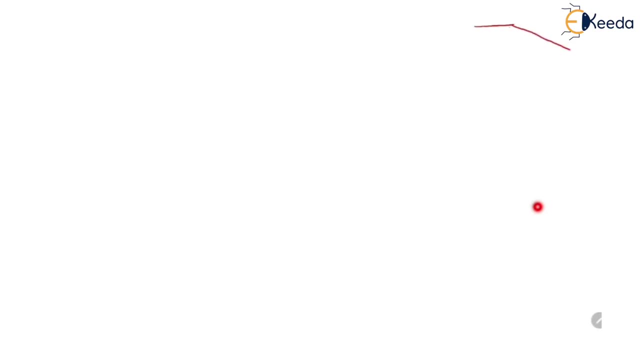 surface is at higher elevation than the actual ground surface. So for this railway track the ground surface is at higher elevation than the actual ground surface. So for this railway track the ground surface is at higher elevation than the actual ground surface. So for this railway track the ground surface is at higher elevation than the actual ground surface. 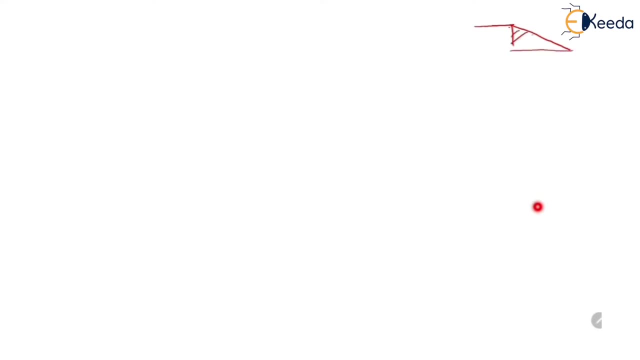 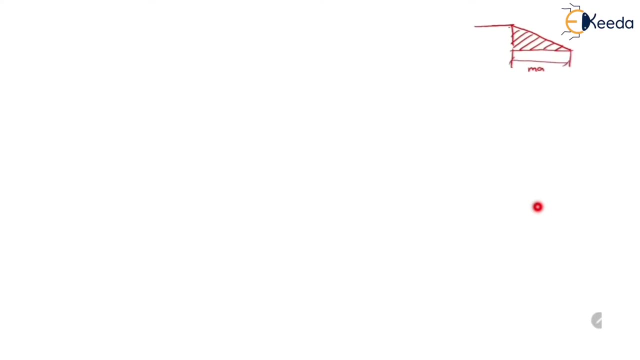 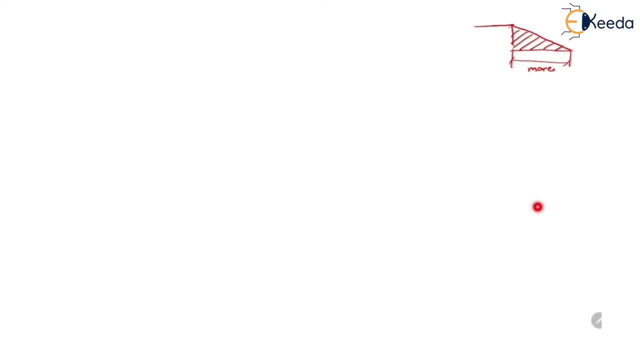 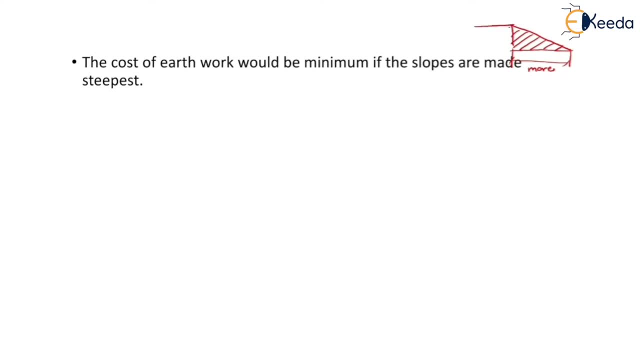 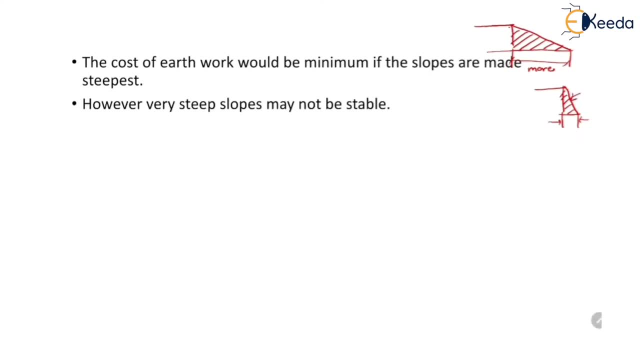 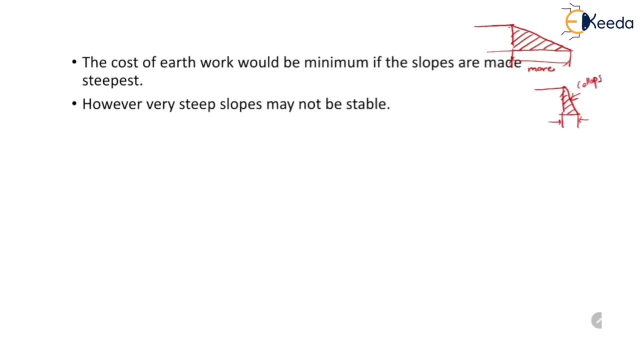 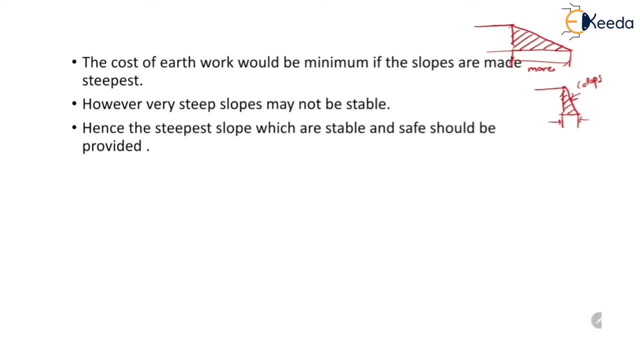 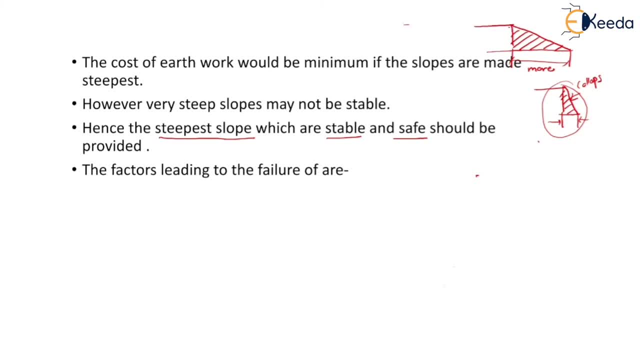 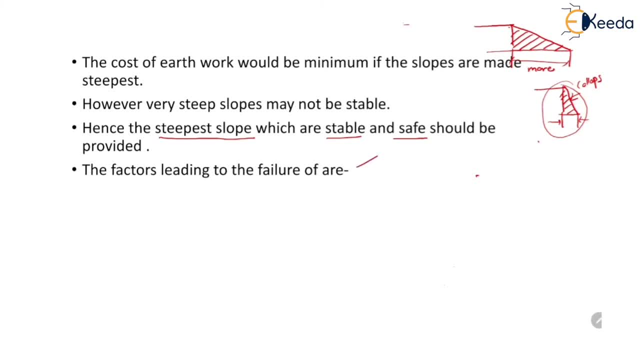 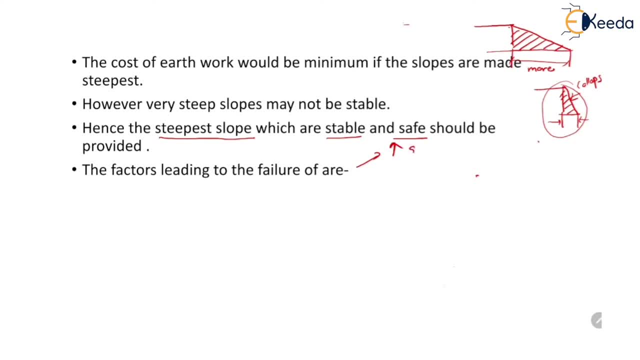 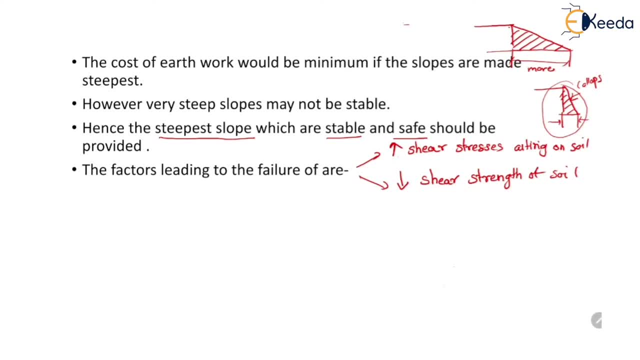 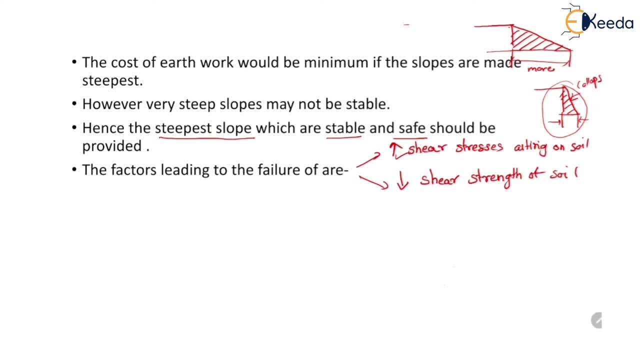 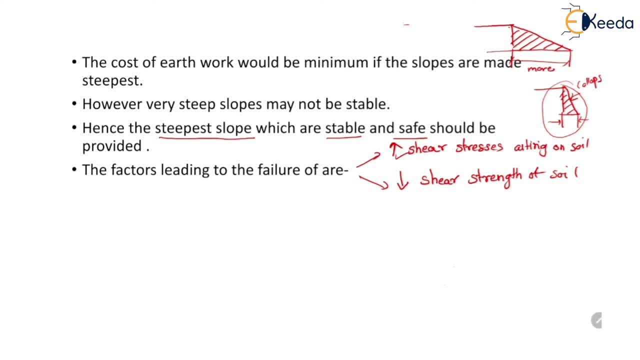 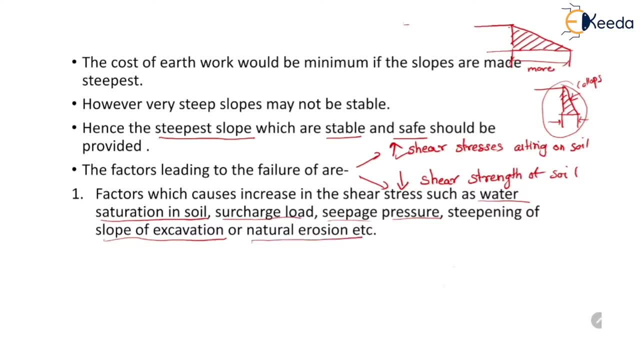 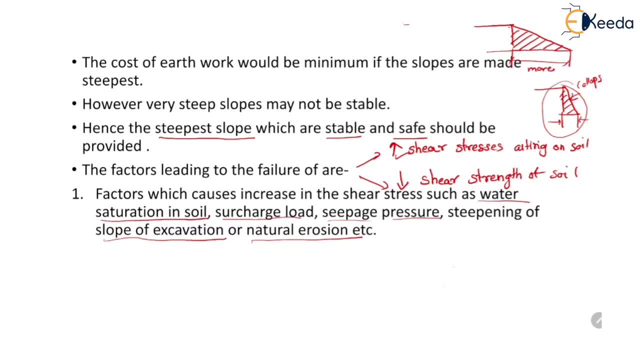 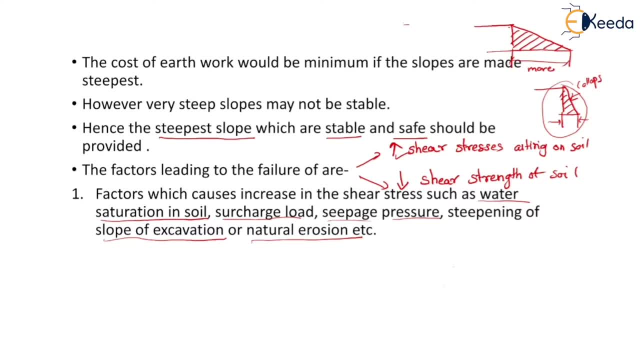 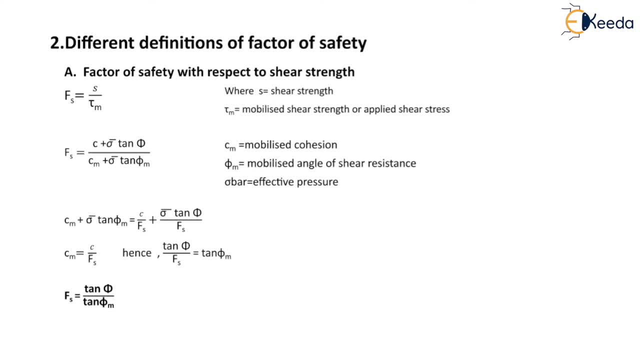 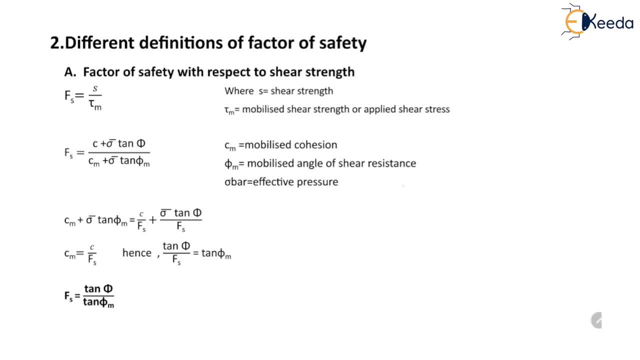 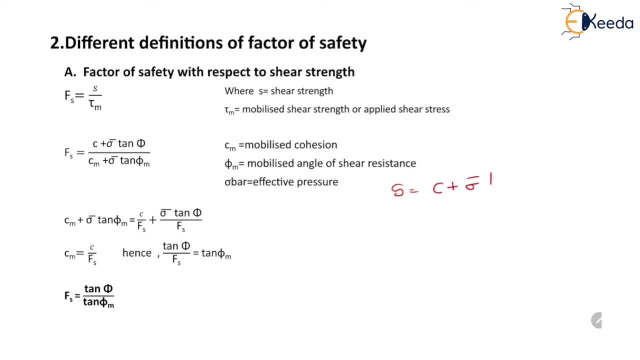 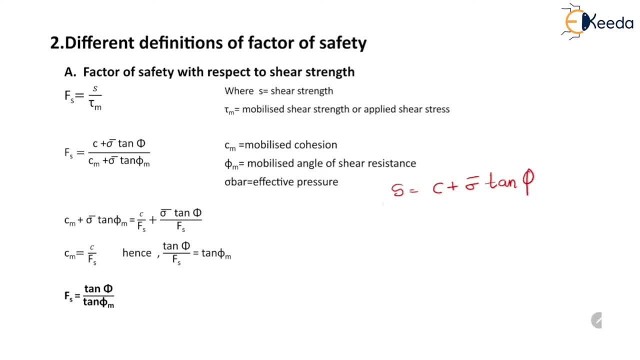 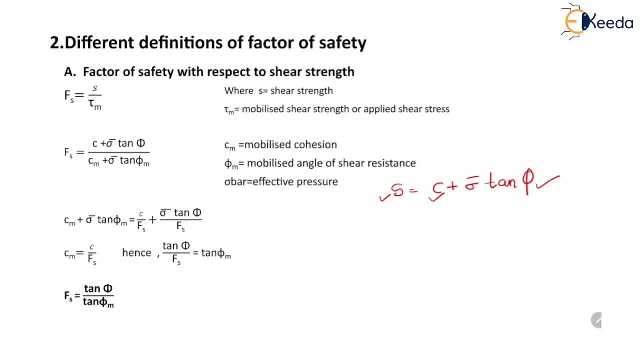 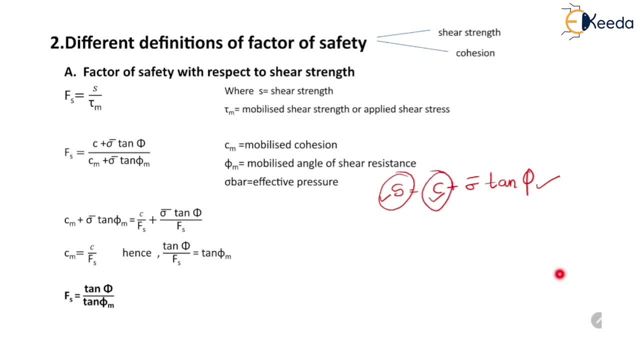 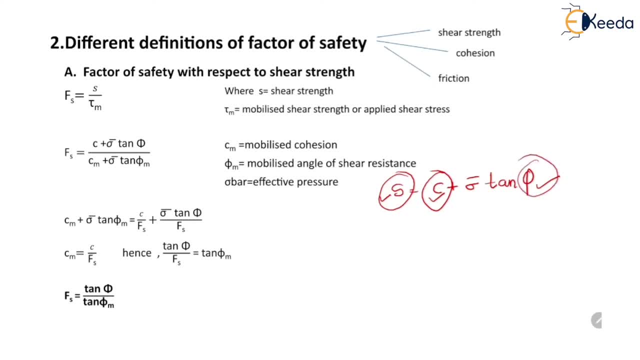 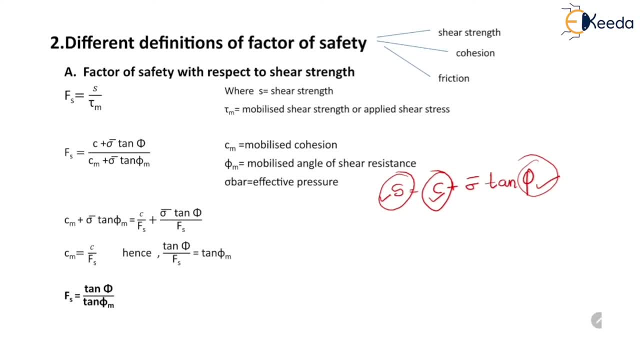 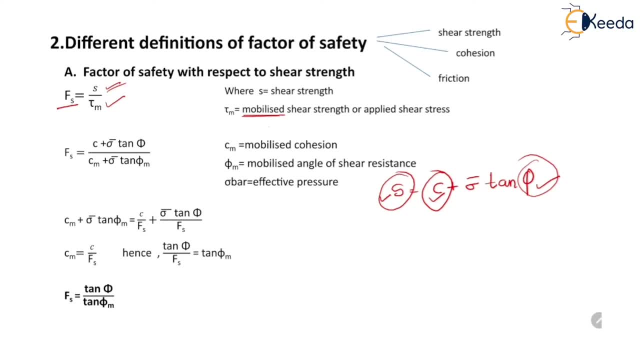 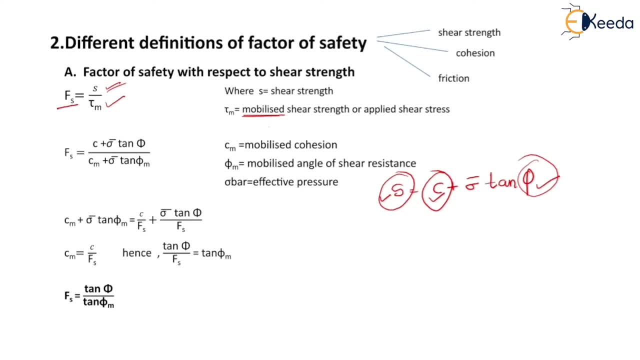 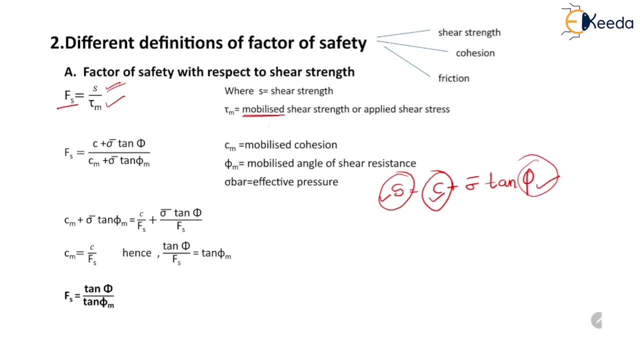 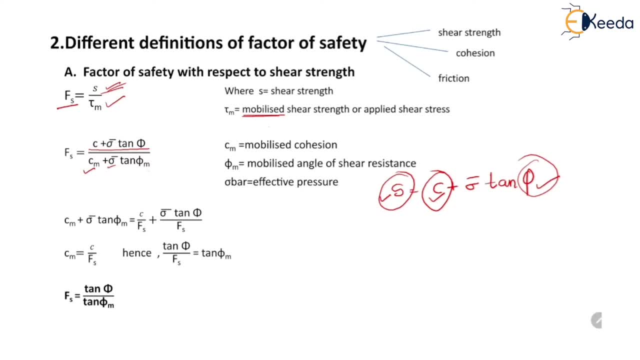 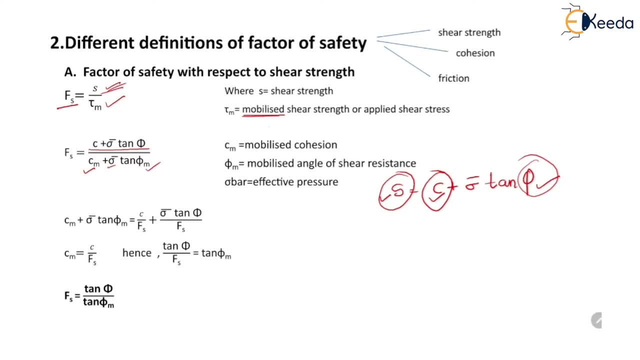 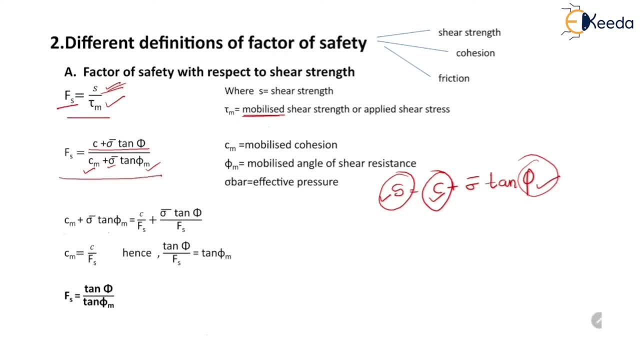 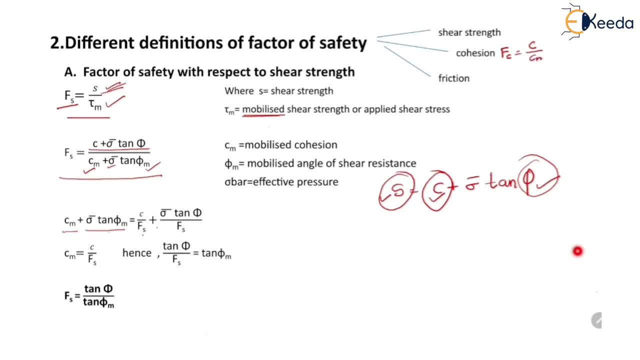 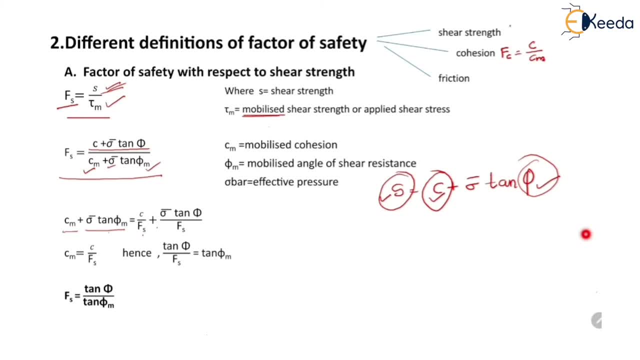 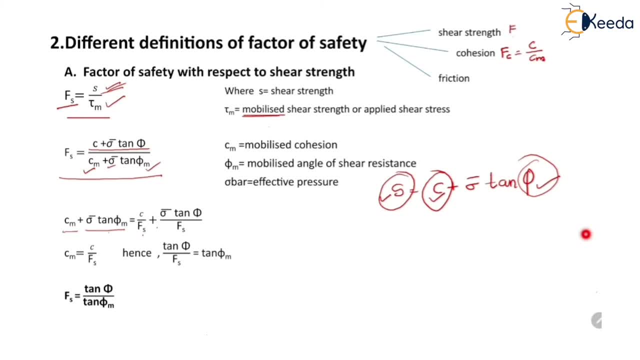 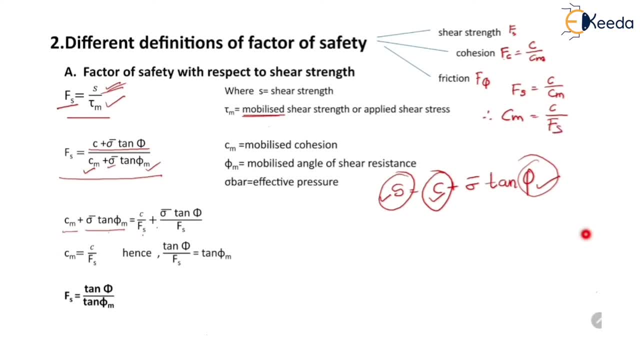 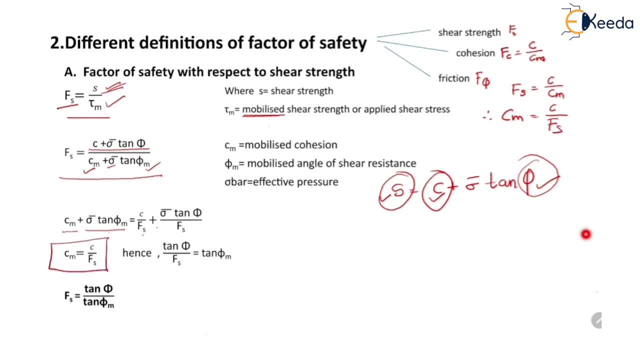 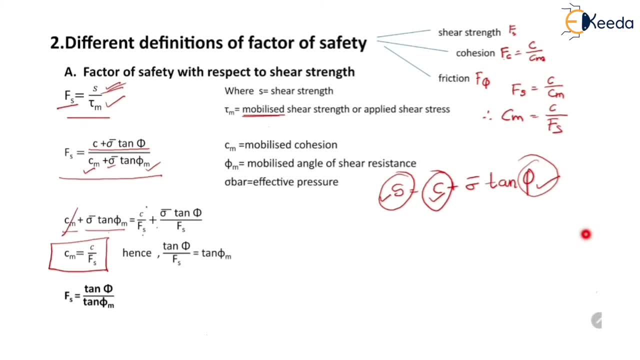 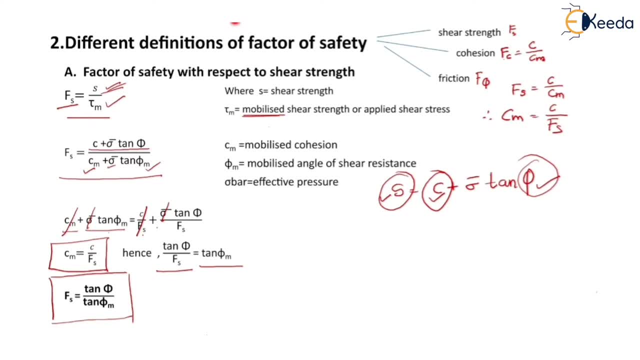 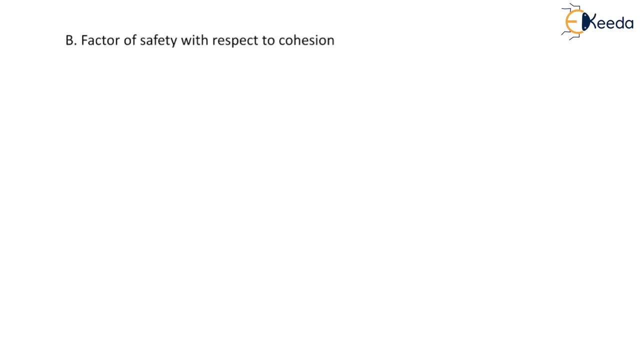 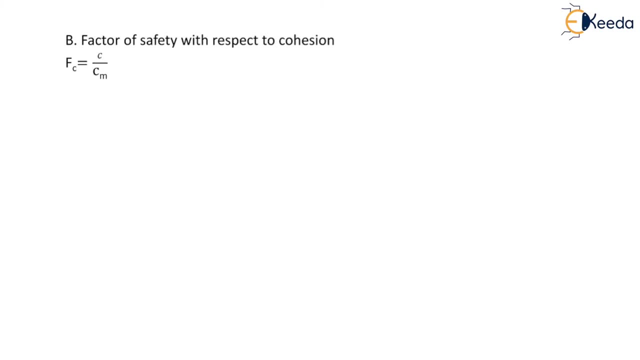 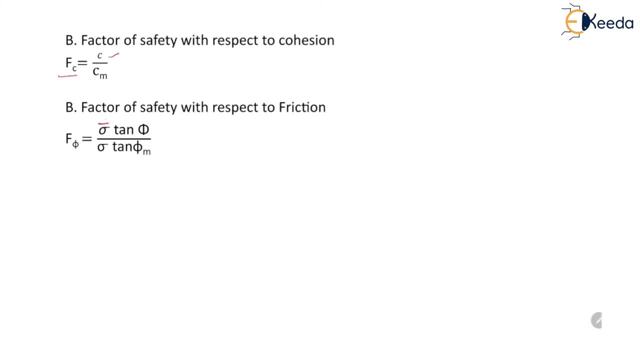 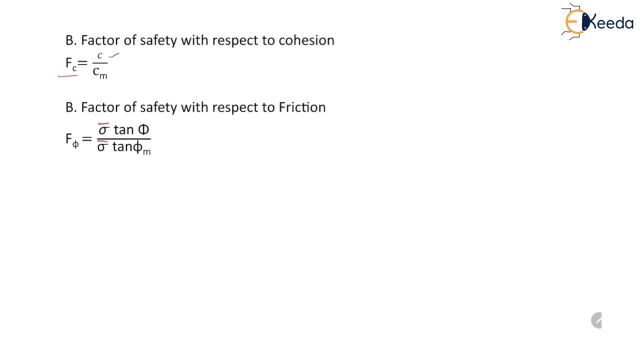 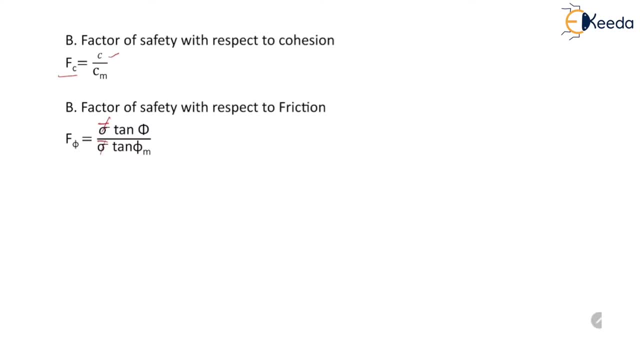 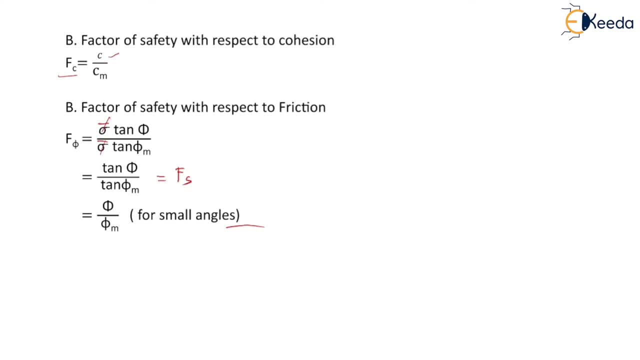 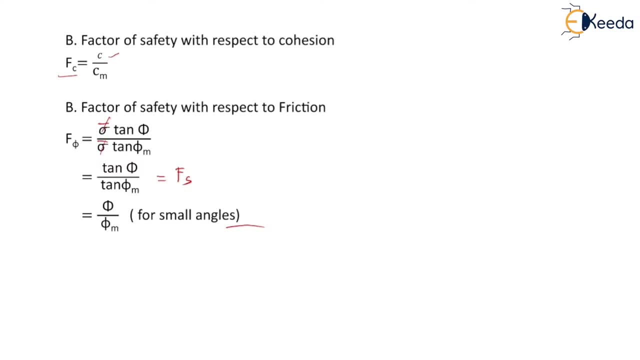 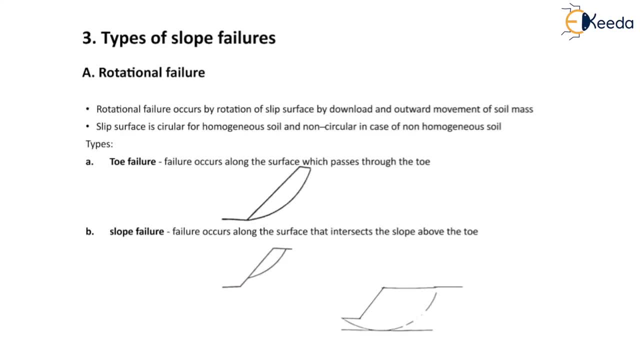 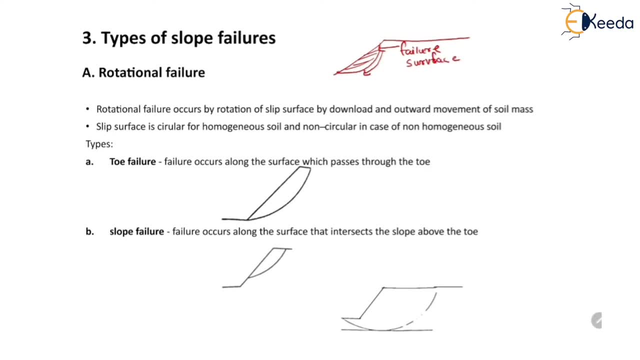 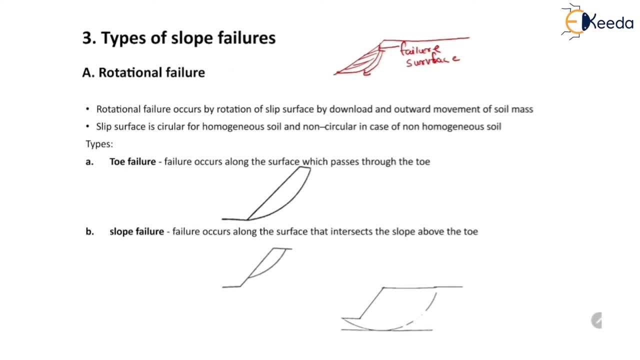 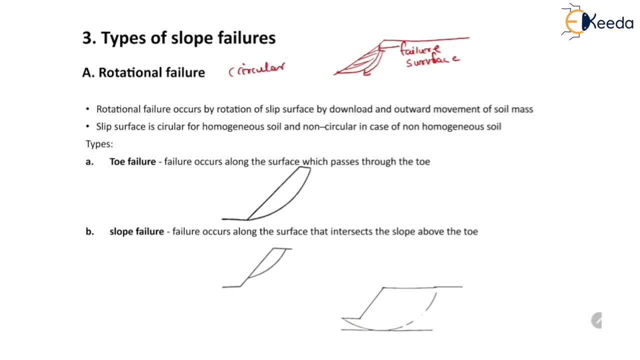 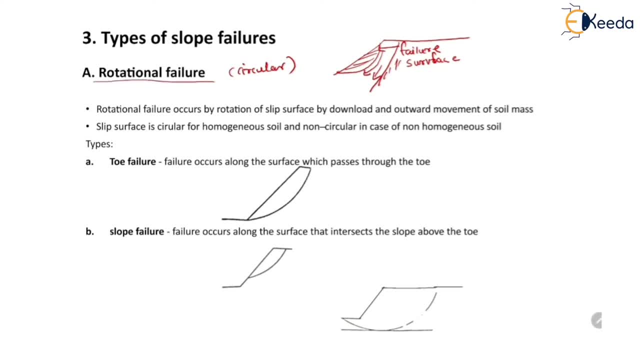 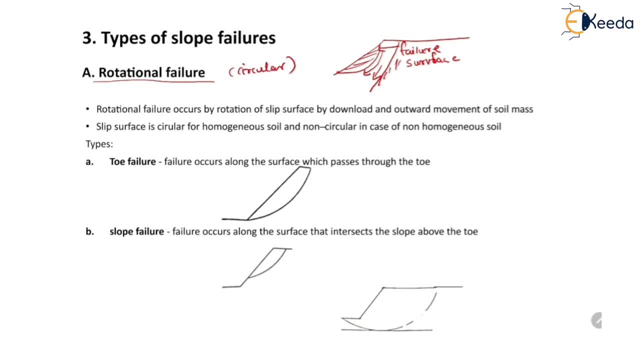 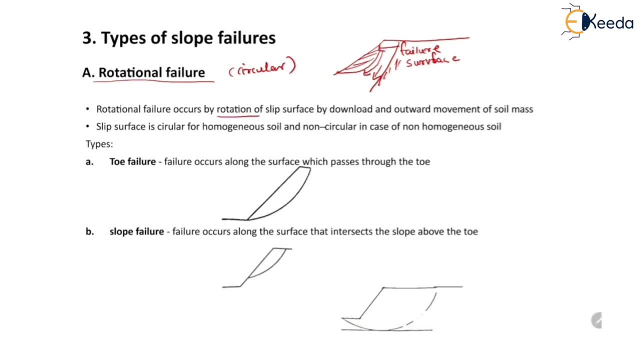 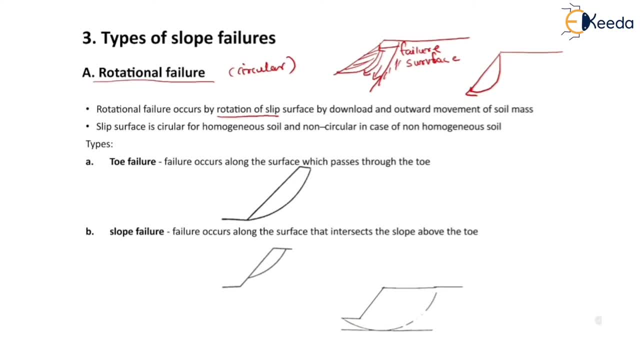 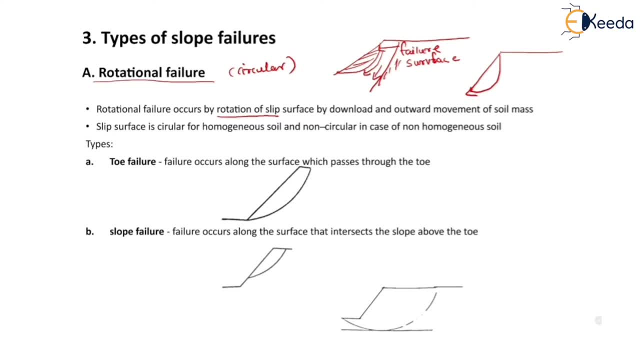 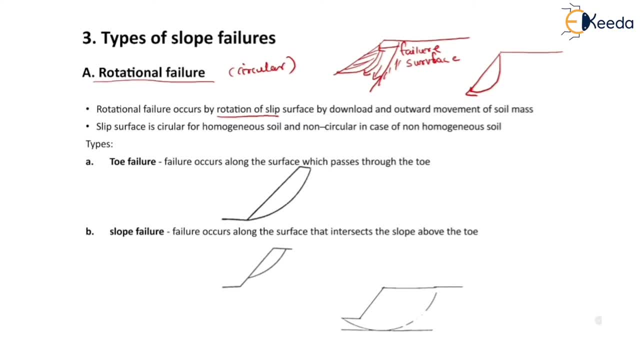 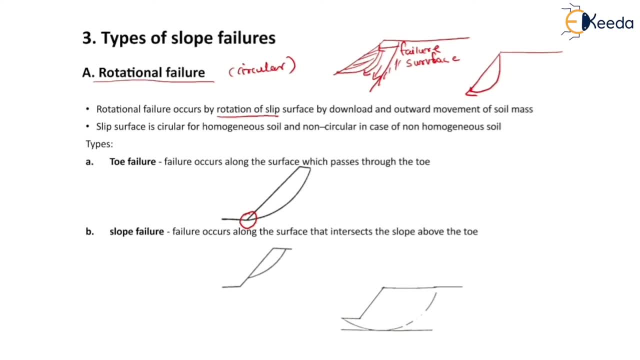 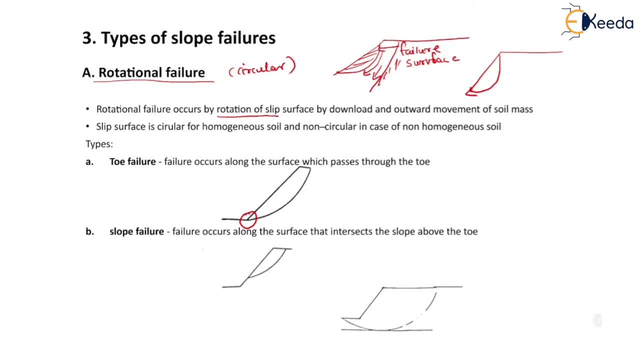 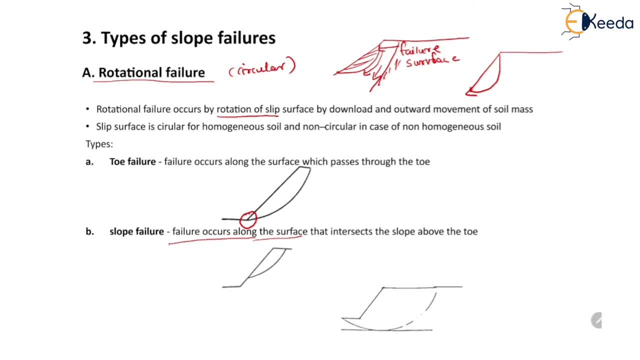 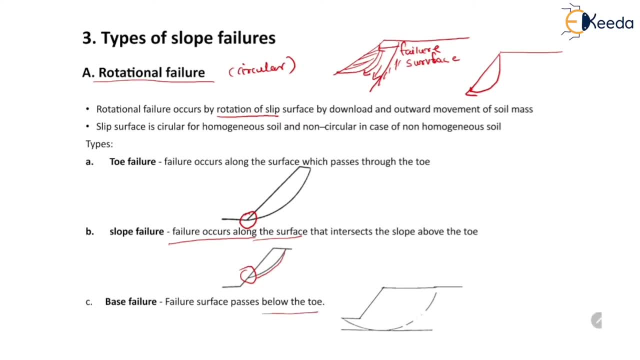 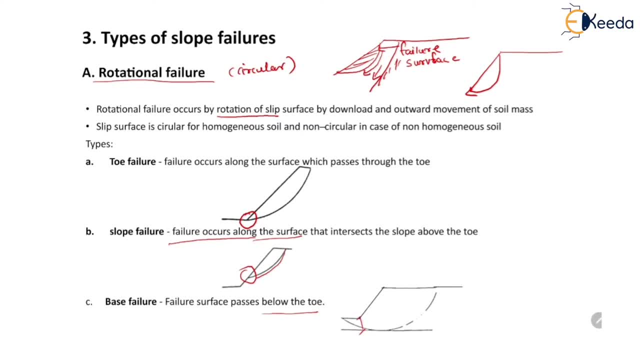 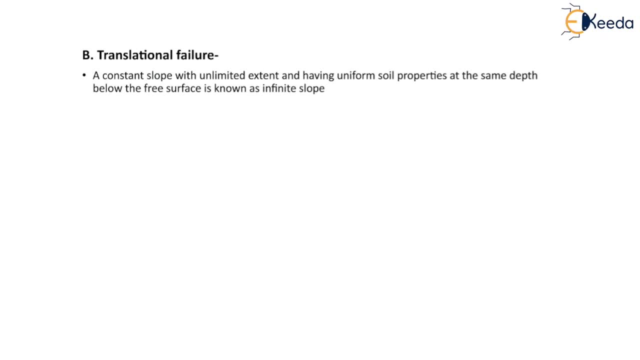 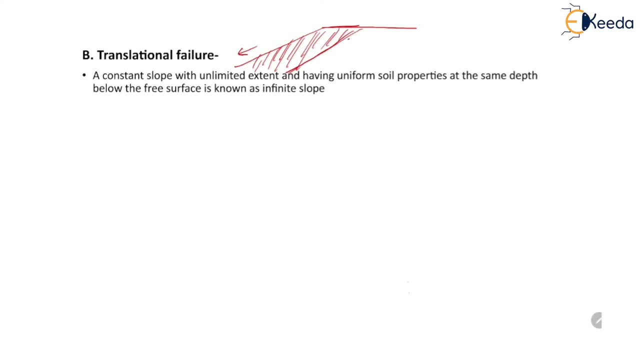 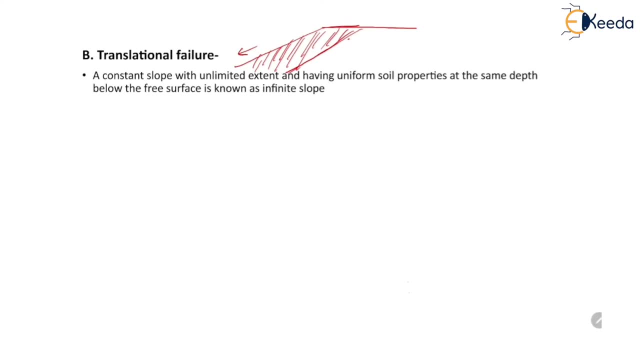 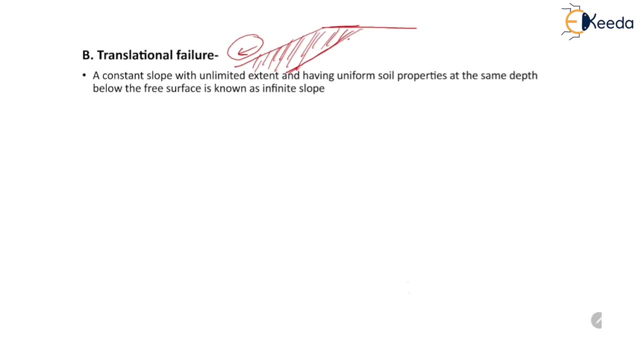 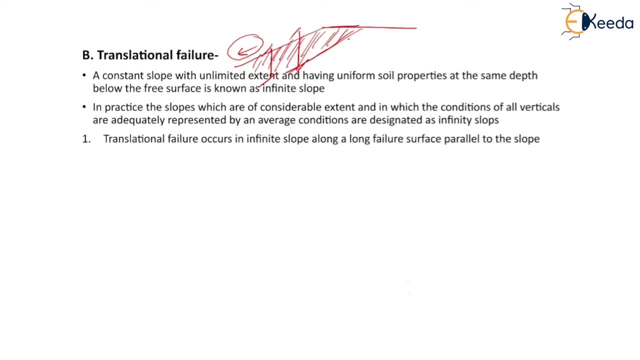 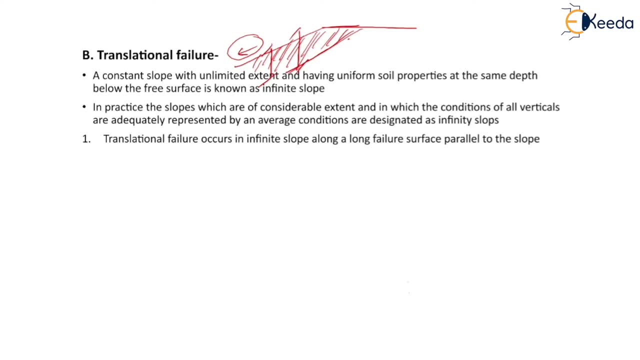 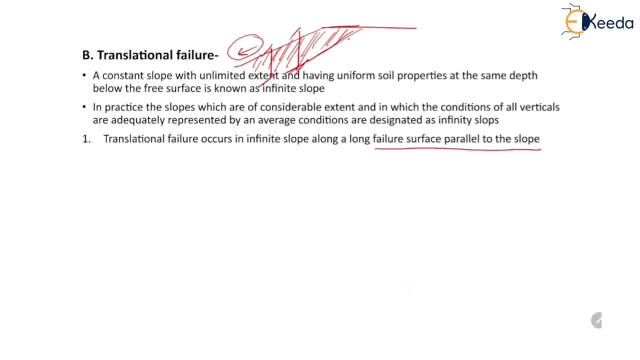 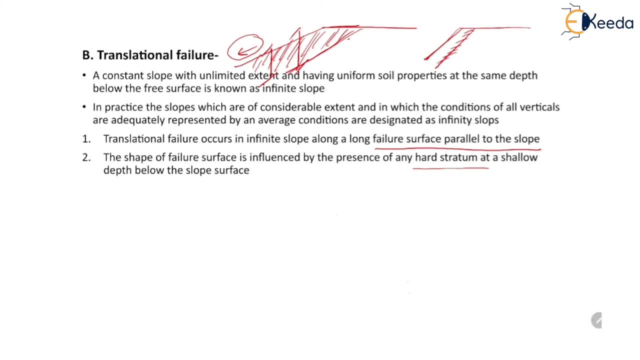 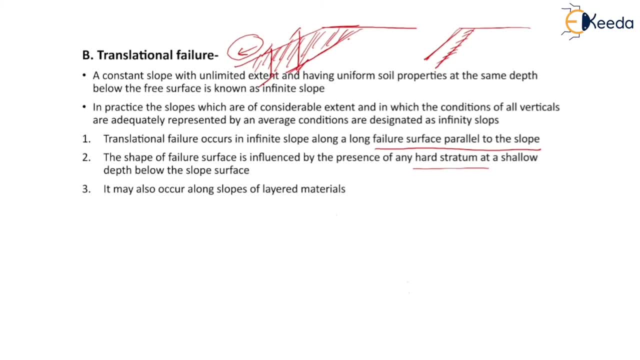 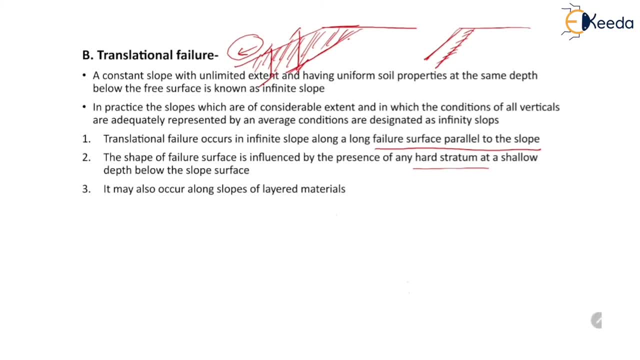 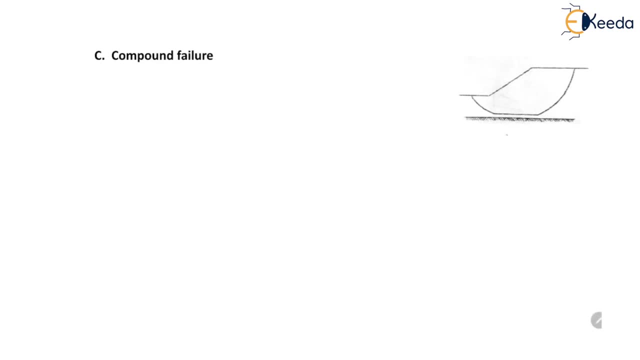 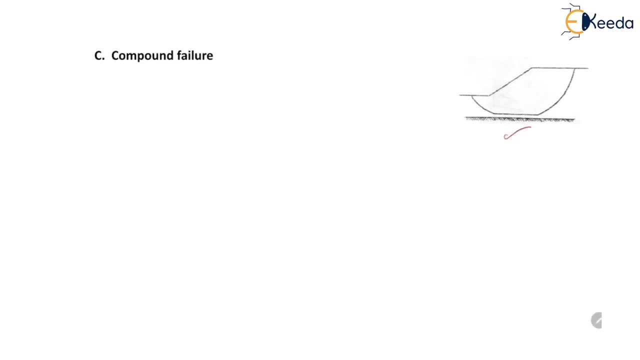 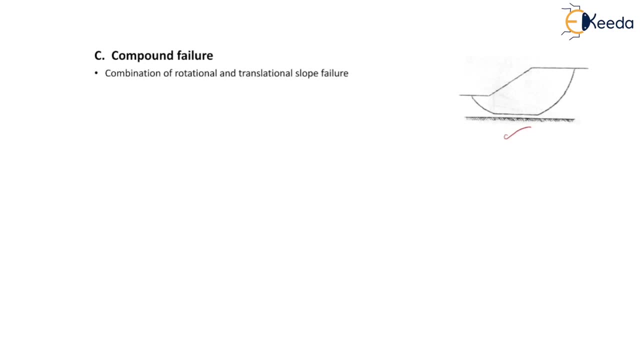 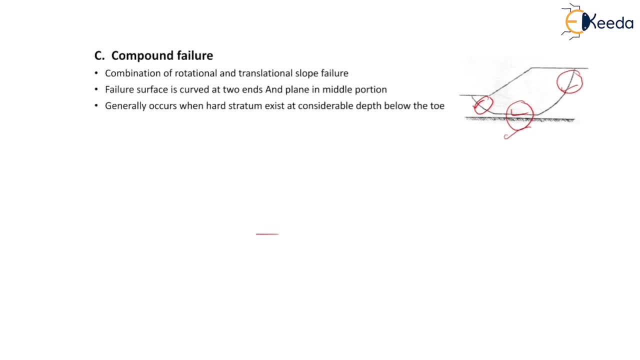 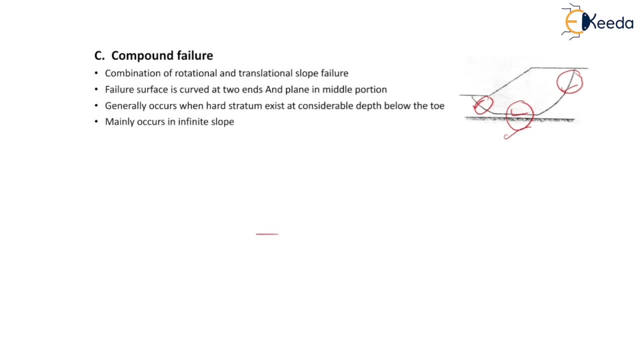 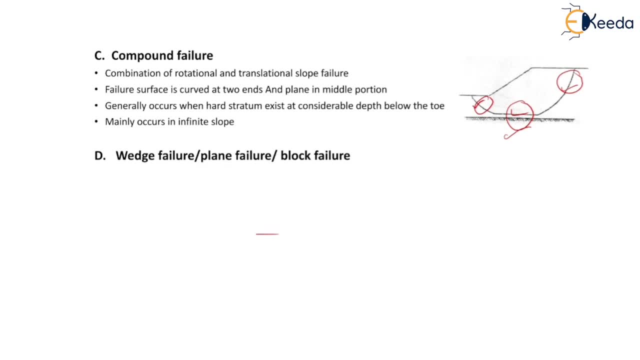 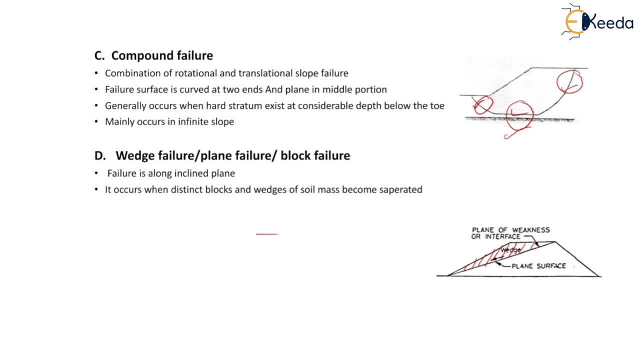 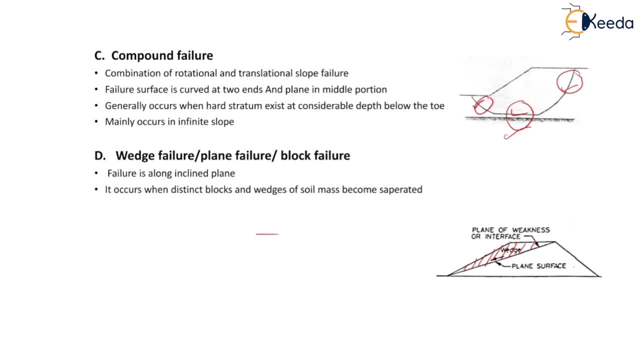 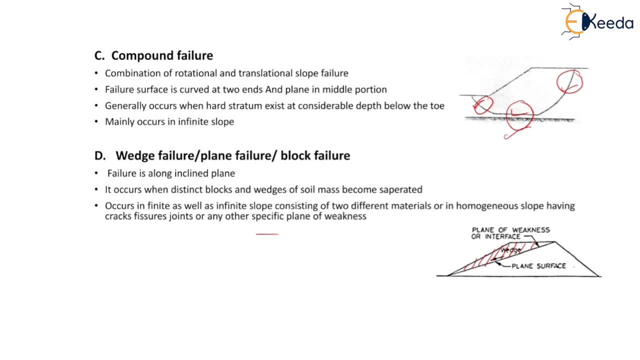 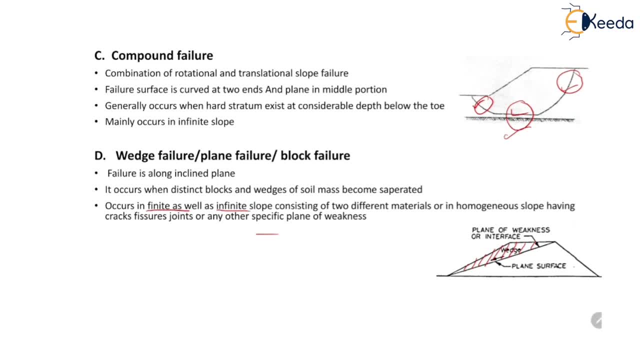 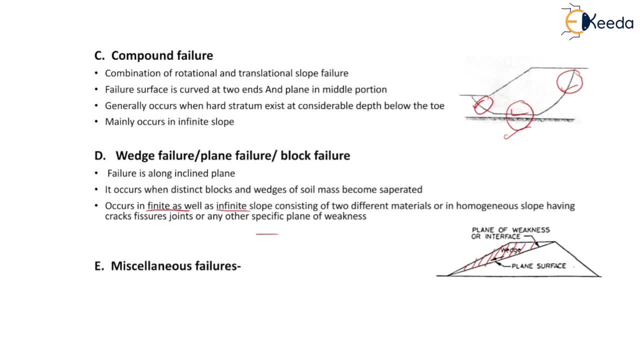 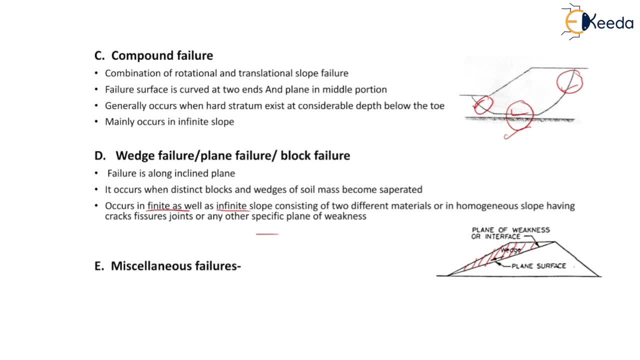 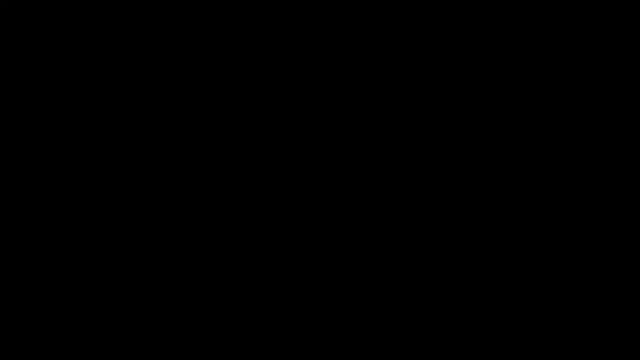 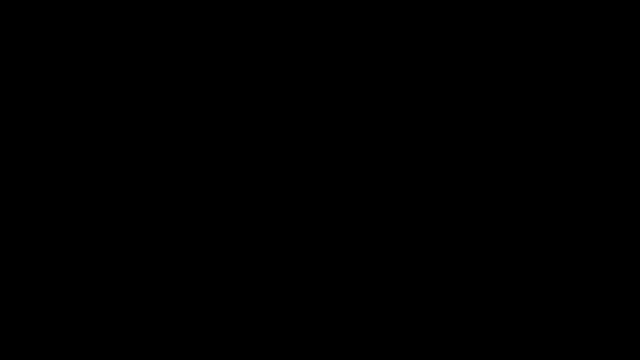 track, the ground surface is at higher elevation than the actual ground surface. So for this railway track, the ground surface is at higher elevation than the actual ground surface. So for this railway track, the ground surface is at higher elevation than the actual ground surface. So for this railway track, the ground surface is at higher elevation than the actual ground. 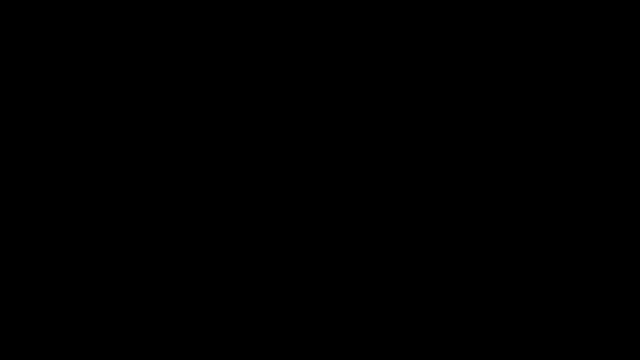 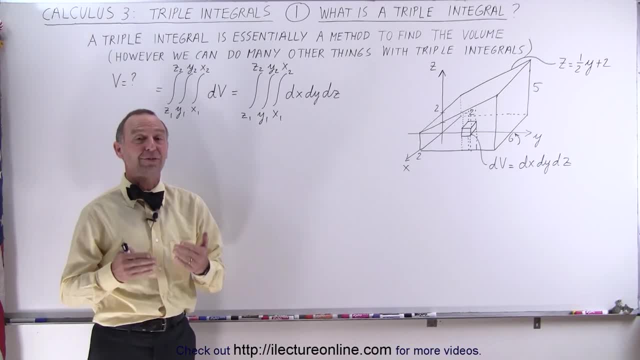 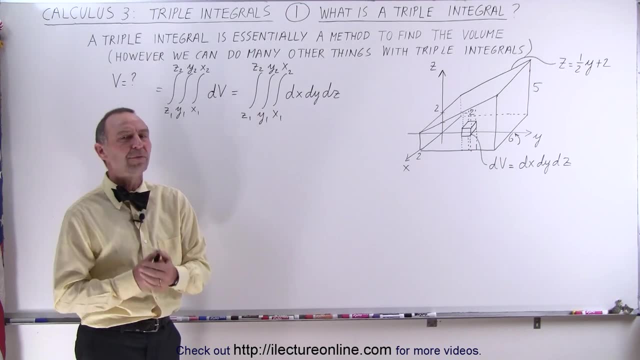 Welcome to ElectronLine. Here's our first video in a series of videos on triple integrals. And the question is: what is a triple integral? Why do we need them? What do we use them for? And essentially, a triple integral is used to find the volume of an object.